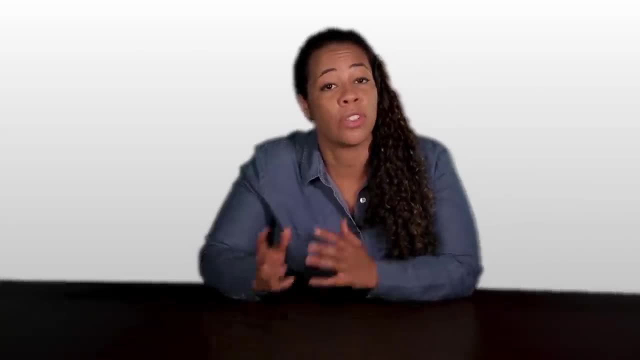 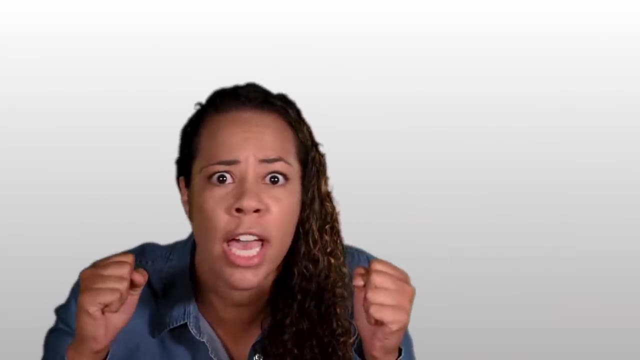 others. You just have to be really passionate about building. People with an associate's degree and on-the-job experience can also become PMs, because, again, it's all about the passion. Nationally, according to the Department of Labor in 2018, the median salary for construction 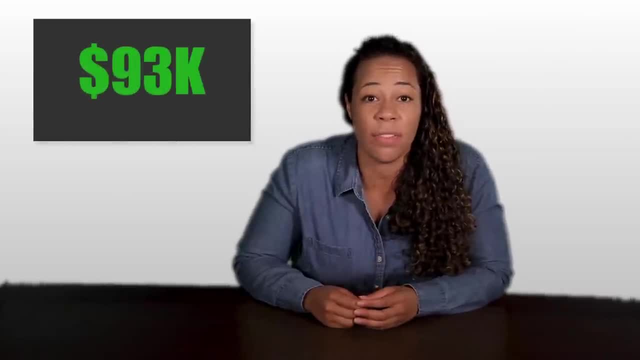 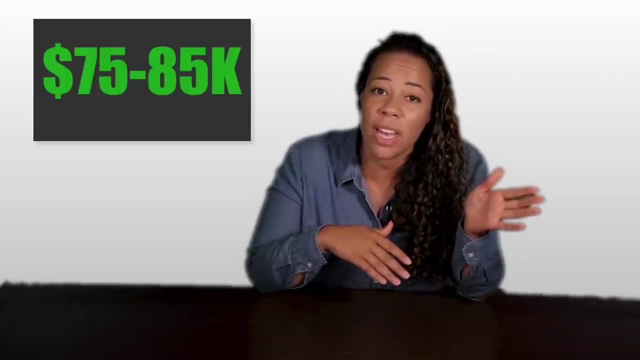 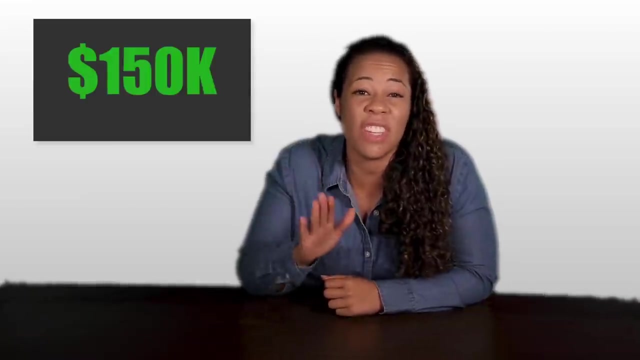 managers is averaged at $93,370.. $93,370.. $93,370.. $93,370. $93,370.. In some regions of the country, entry-level construction managers earn $75,000 to $85,000 with a full benefits package. Experienced project managers can earn $150,000. or more per year. The Department of Labor also said that the job market is expected to go up 11% by 2026.. Some of the mega projects have several layers of project managers, including junior and senior PMs, as well as project executives. 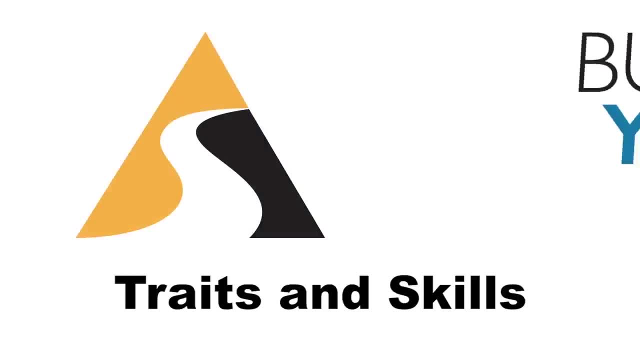 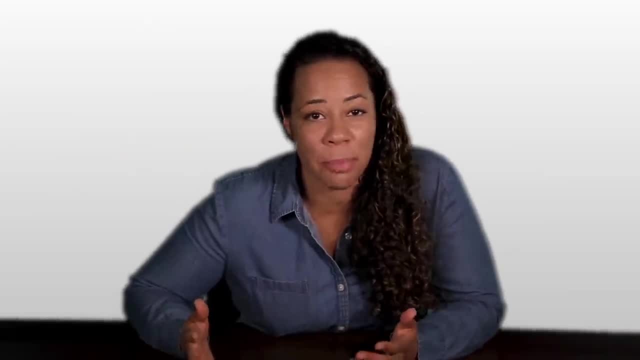 No doubt ICEBET's talent seems to be making headlines for many partankeners as well. To tell you a story, at the beginning of the year I introduced, Being a good communicator is probably the most important skill for a PM to have. 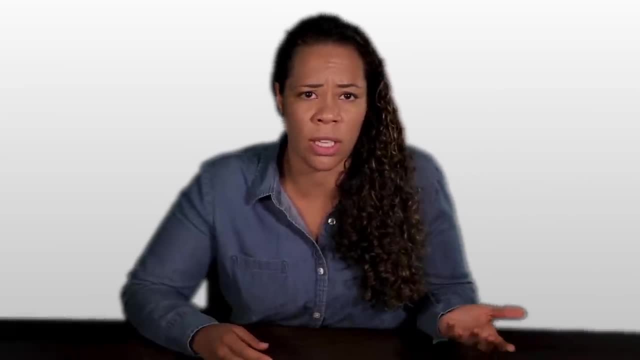 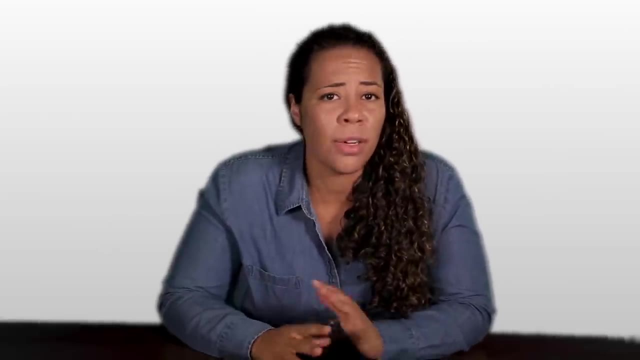 You're going to be dealing with a variety of positions, from corporate-level CEOs to brilliant engineers that talk and technobabble. Project management usually means a lot of in-office work. There are tons of meetings, phone calls and lots of time behind a computer. 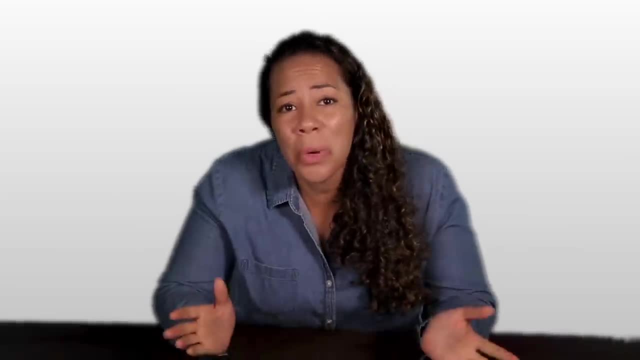 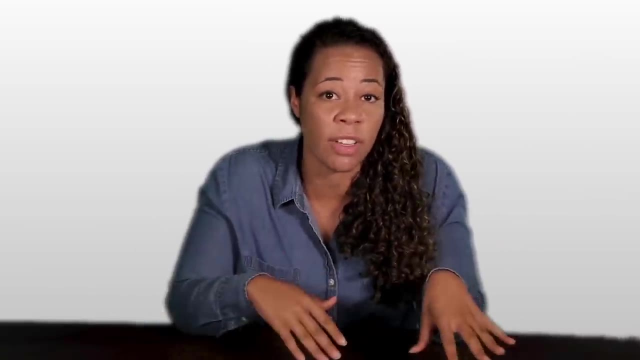 If the thought of sitting in an office all day makes you cringe, don't worry. there's still plenty of time spent on-site. At the entry-level positions, you'll probably spend more time at the job site than in an office. As your career advances, however, you will spend more time in the office than in the 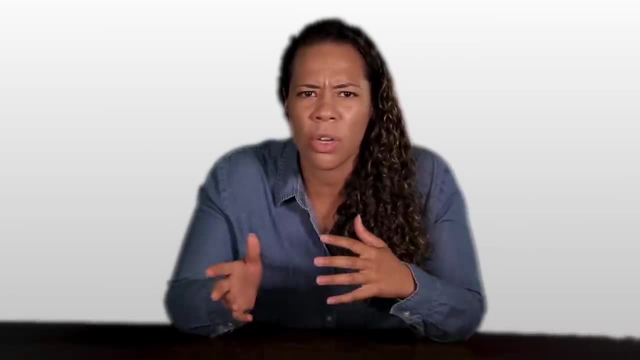 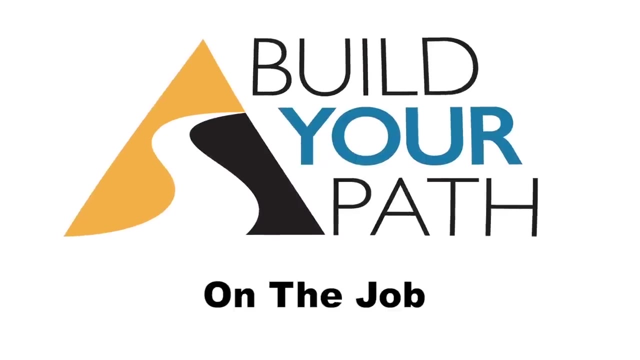 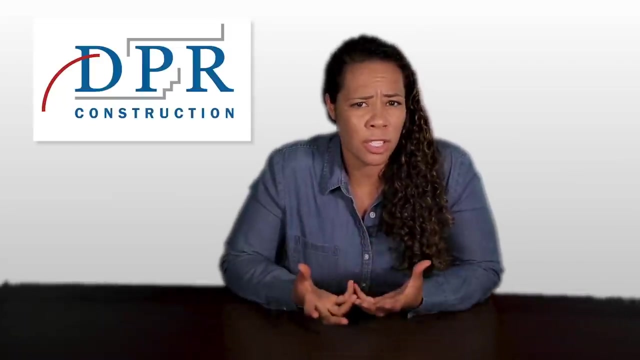 field. There isn't much physical building going on in this career track, so if you're someone who enjoys working with their hands or like to be outside all day, other career tracks may be for you. And now some knowledge from our sponsor. Being a project manager sounds really easy. 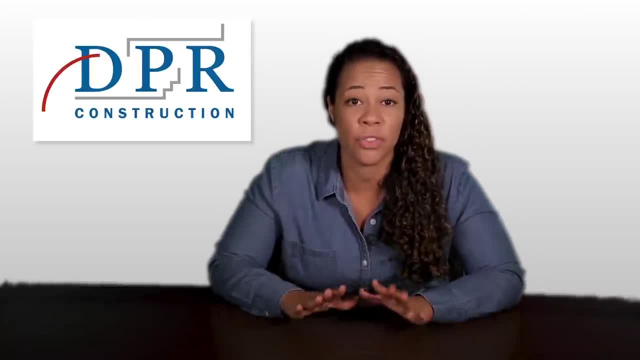 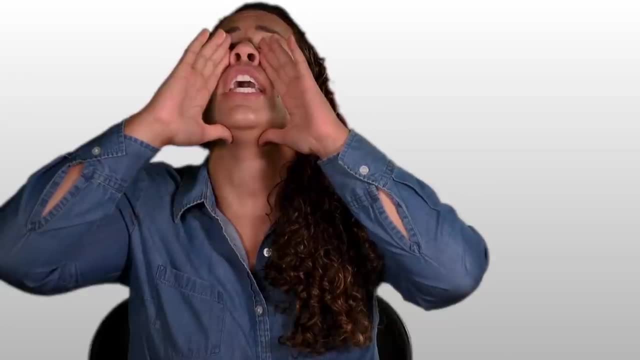 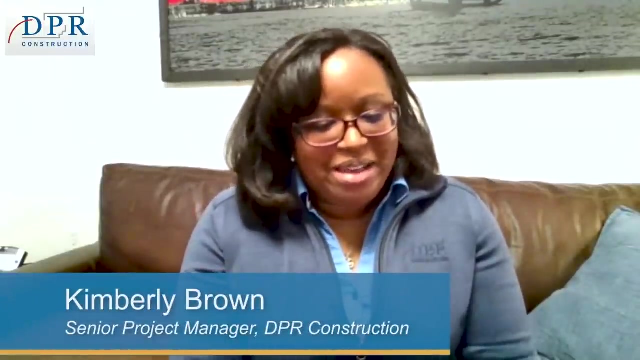 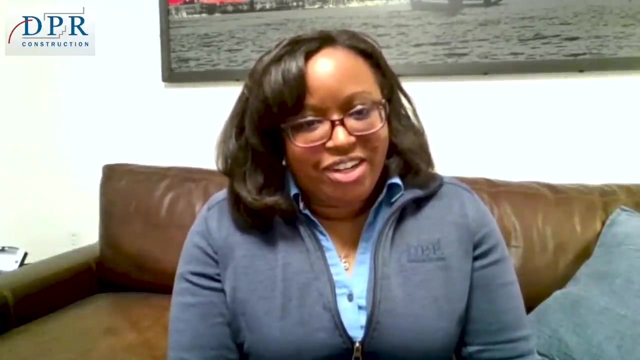 Really intimidating. But our wonderful sponsor was nice enough to give us some first-hand PM experience, So you know what that means. FIELD TRIP Construction management is awesome Why? Because every day you learn something. There's always a challenge you need to conquer. 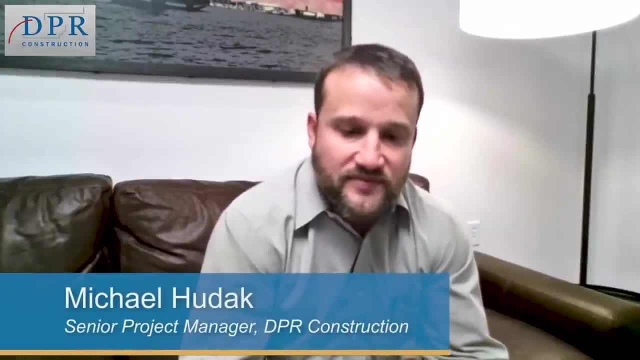 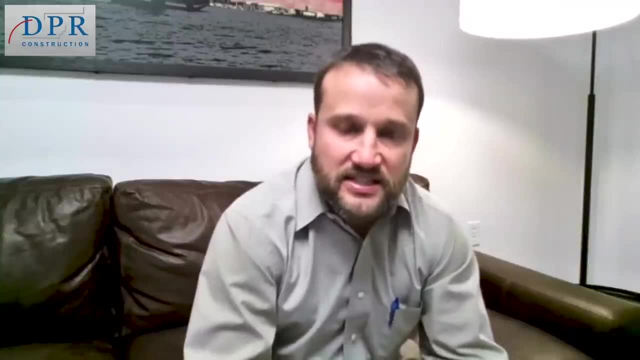 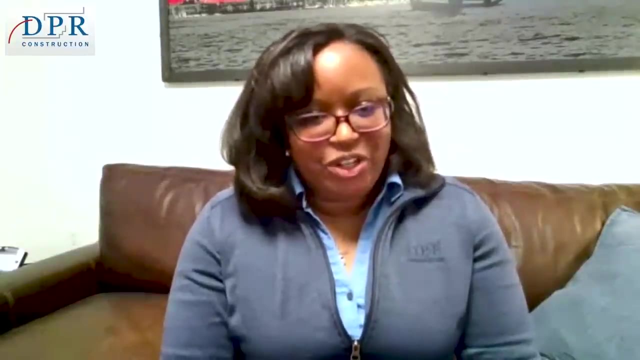 You can wake up on a Tuesday and be faced with a whole new, different set of challenges. So if you like the flexibility and the kind of change in scenery and it's kind of something new every day, this could be the field for you. The days always start early: 6.30,, 7 o'clock in the morning. 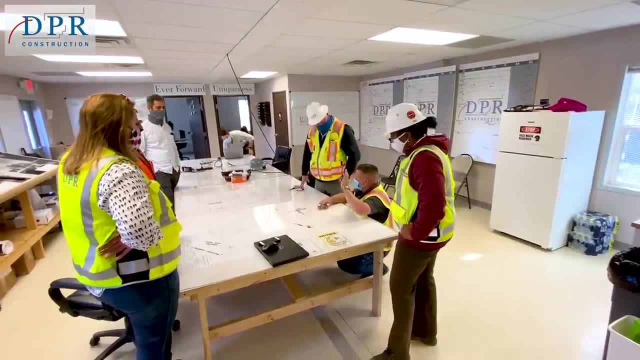 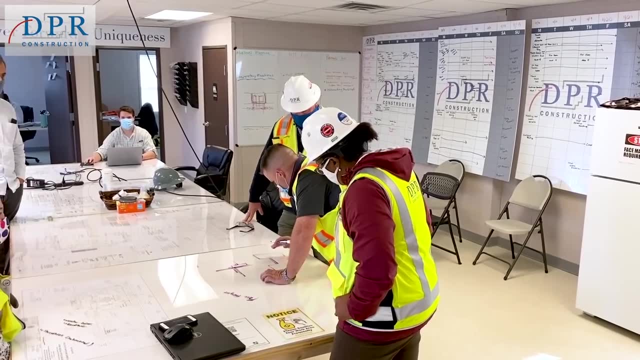 And you always start with a huddle with your subcontractors to kind of see what their goal is for the day, what their plan is for the day. Typically in the morning is when you get all of their issues and things are trying to work out. 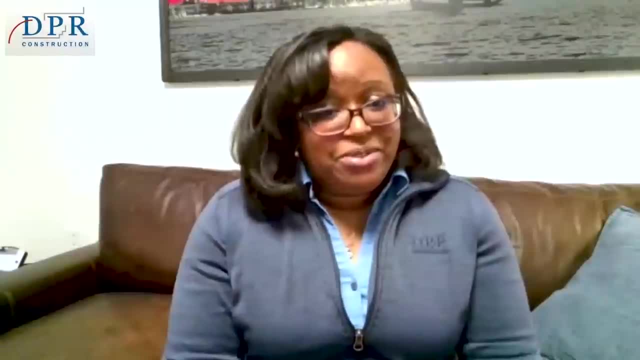 So you may be able to resolve those issues with them in the field. But if you don't, you're not going to be able to do it Or you may have to take those issues back to the design team or to your team to help. 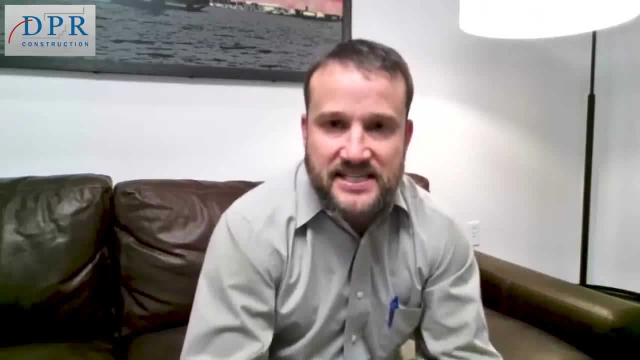 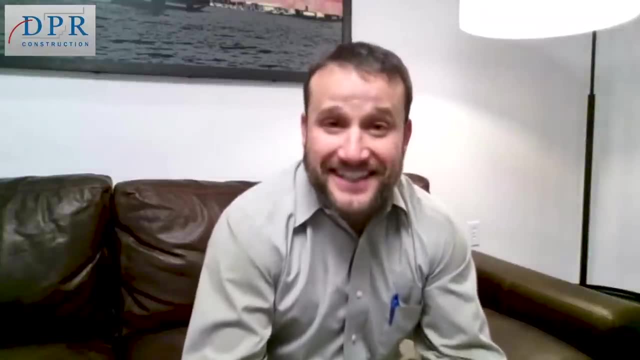 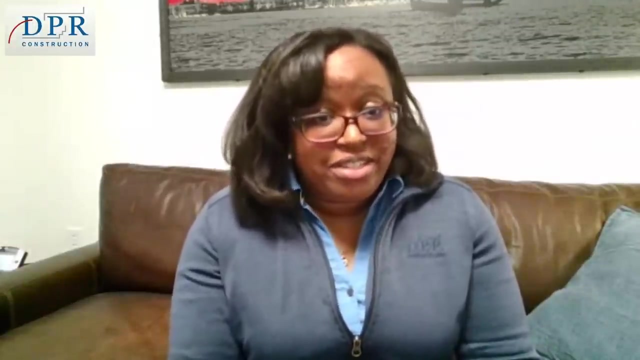 figure it out. What we do on a day-to-day basis is essentially getting other people to do what we need them to do when we need them to do it, when they're not necessarily interested in doing it at that time. So in construction management, you have a design team, you have the construction team. 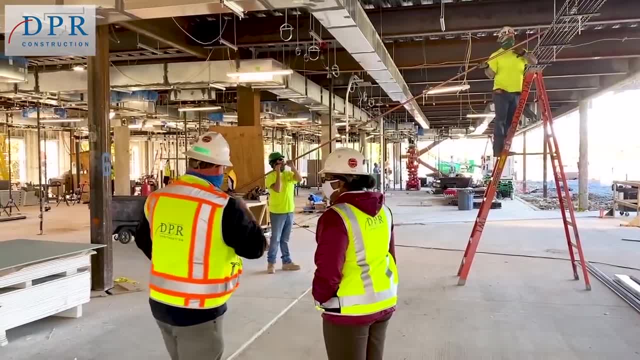 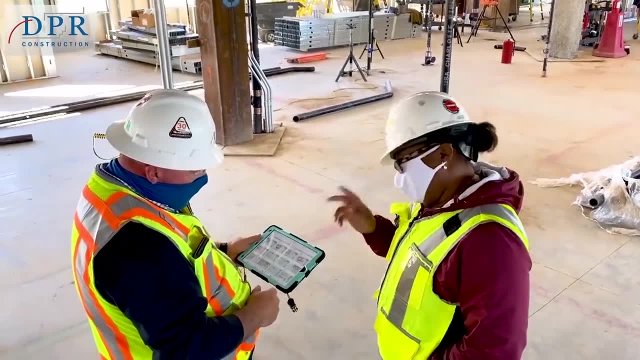 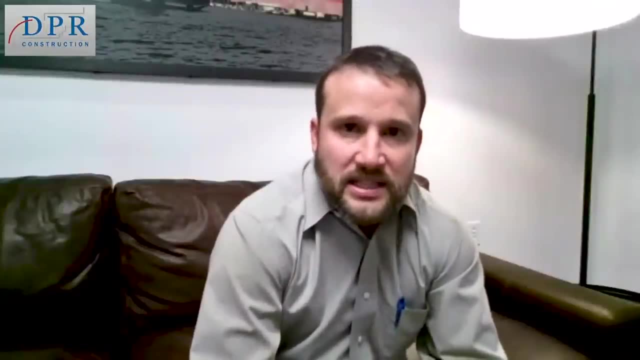 you have the trade partners or the subcontractors that specialize in their own scope, And all of those individuals have to come together to make the project happen And it really takes teamwork. So I appreciate and I enjoy the problem solving and the collaboration. It's also a very rewarding and satisfying career because you get to touch something. 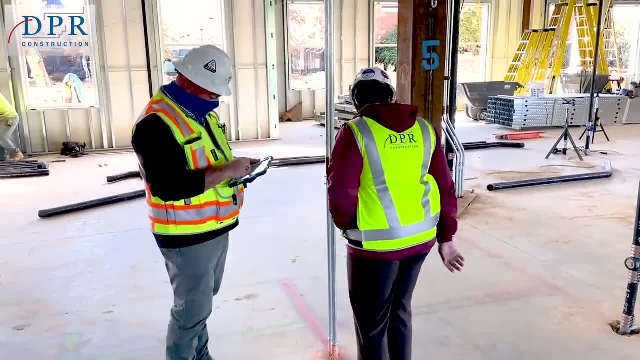 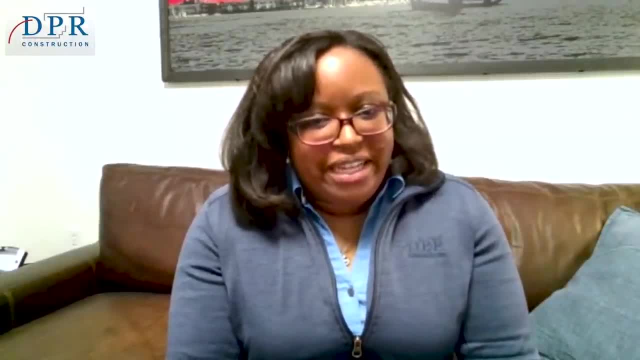 tangible. A lot of young people are really anxious to get out there and get their feet dirty. Internships are the way to go, because you have a chance to get your feet dirty, really get in the grind and understand if this is really what you want to do and have an impact too. 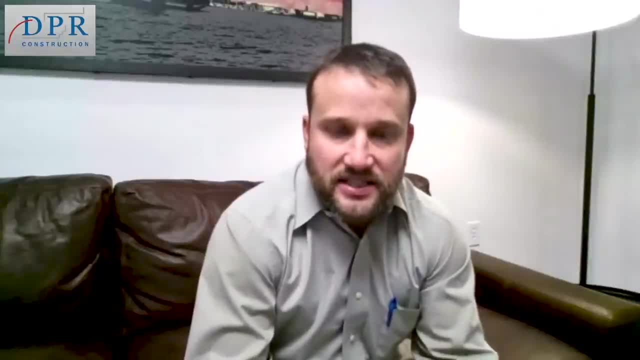 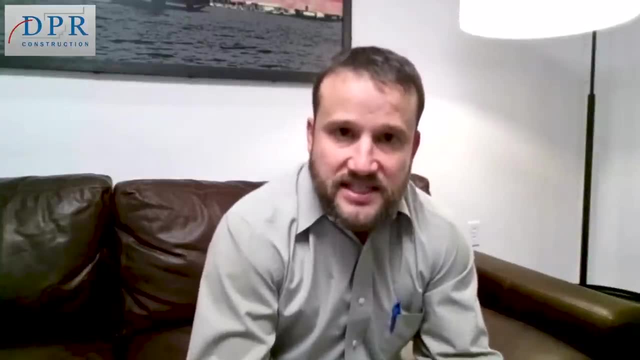 because we give interns real work. The typical pathway to getting in the construction management is really one of two ways. right, You can come up through the trades and develop a skill set and stay in the field. if you will, you know the superintendent route. 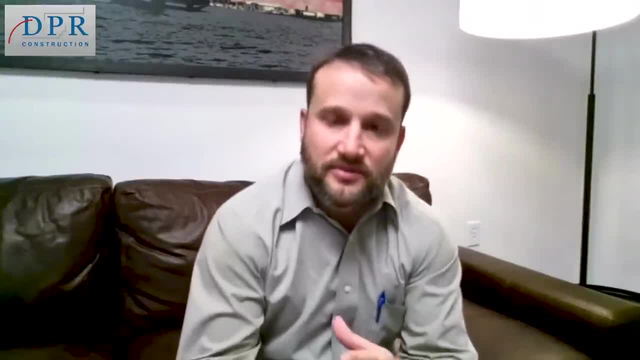 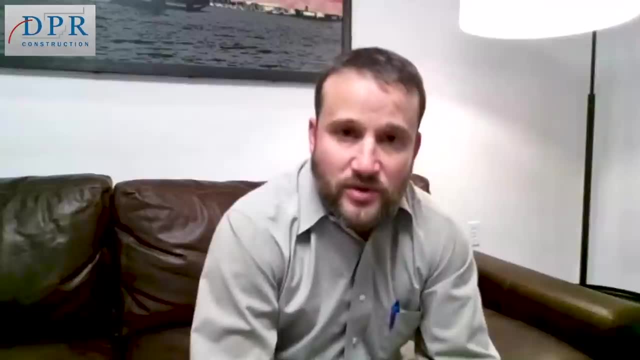 Or you can also stay in the office through the project engineer route, through the project manager route, And that is typically, more often than not, achieved by Attaining your four-year degree, Whether you want to build homes, whether you want to be in the commercial aspect and build.